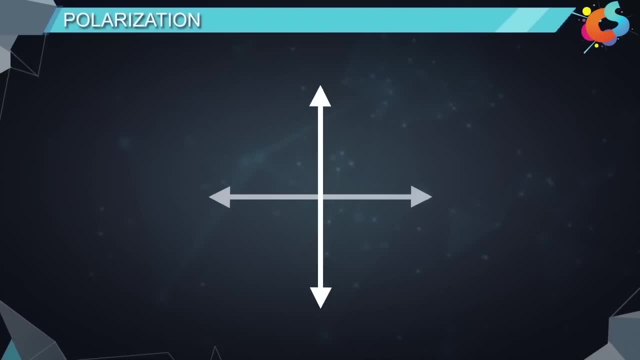 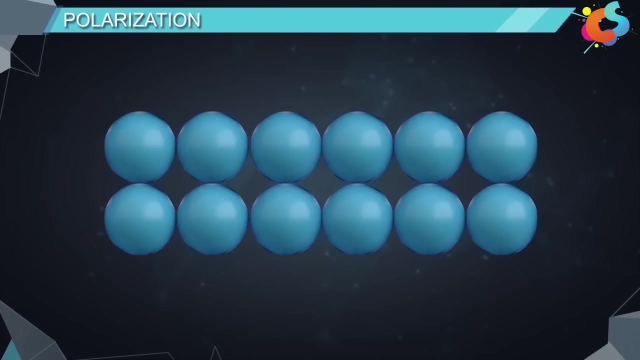 oscillation. The oscillation can be in this direction, this direction and even in this direction. We know that electromagnetic waves are produced by excited atoms. A particular atom may produce electric field vibrations in this direction. Its neighbor may be the same atom. Similarly, different atoms of a material can produce vibrations in variety. 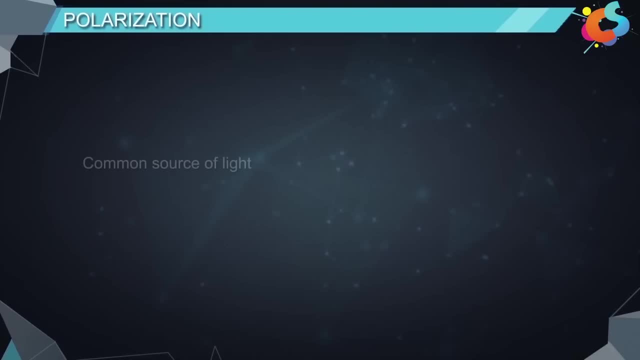 of directions. Due to this, a common source of light like incandescent bulb, candle, flame, fluorescent lamp, etc. emit light that have electric field vibrations in a number of directions. This type of light beam, which has vibrations in more than 1.5 degrees, can produce vibrations. 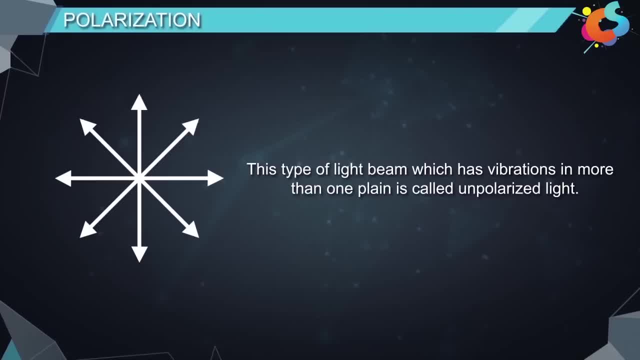 in a variety of directions. This type of light beam, which has vibrations in more than 1.5 degrees, can produce vibrations in the direction of light. This type of light beam, which has vibrations in only 1 plane, is called unpolarized light. Similarly, a light beam which has vibrations 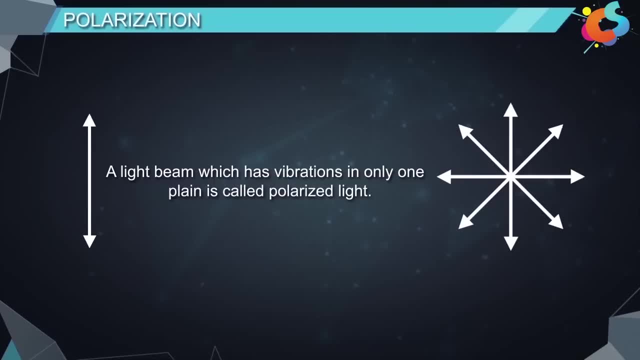 in only 1 plane is called polarized light. The electric field vectors in the unpolarized light can be resolved into vertical and horizontal components. Now, this is the simpler way of representing an unpolarized light. However, this is only a front view of the wave. On the side view, the wave is represented in this way Here. 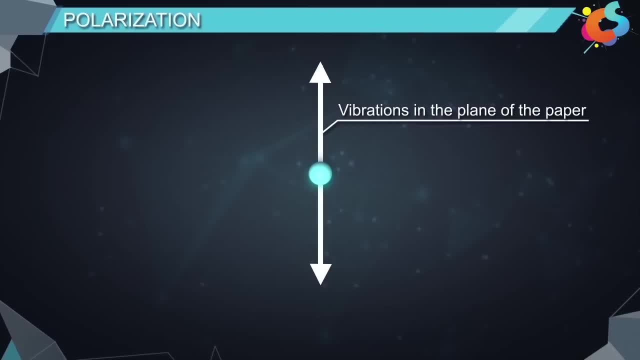 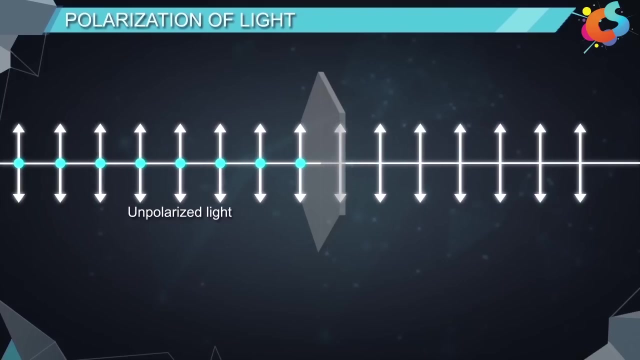 the arrow represents vibrations in the plane of the paper and the dots represent the vibrations in the direction perpendicular to the plane of the paper. Polarization of Light. When an unpolarized light is allowed to pass through a polaroid, let's call it as a polarizer. out of all the vibrations of light, only those vibrations. 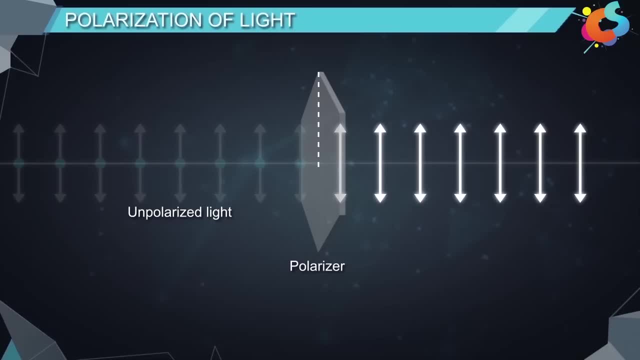 pass through the crystal, which have vibrations parallel to the crystallographic axis. Here the crystallographic axis is represented by the dotted line. Now, the emerging light is a plane polarized light. It contains vibrations in only one plane. The phenomenon of restricting the vibrations of light to particular plane. 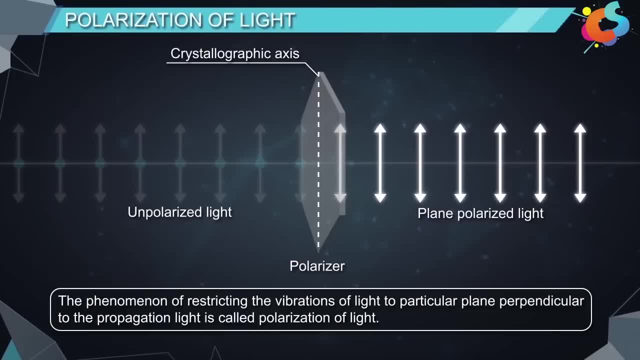 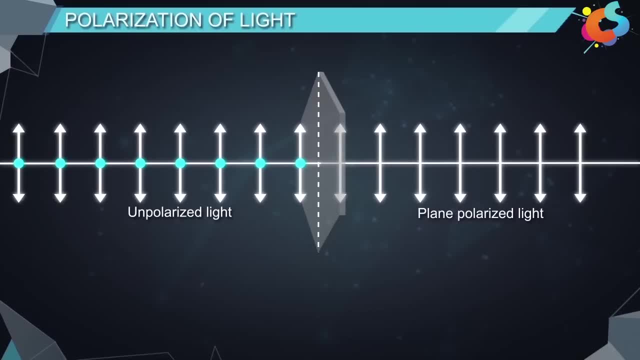 perpendicular to the propagation of light is called polarization of light. Now let us learn about two important terms used in this topic. 1. Plane of vibration- The plane ABCD here that contains vibrations of the plane, polarized light is called plane of vibrations. 2. Plane of 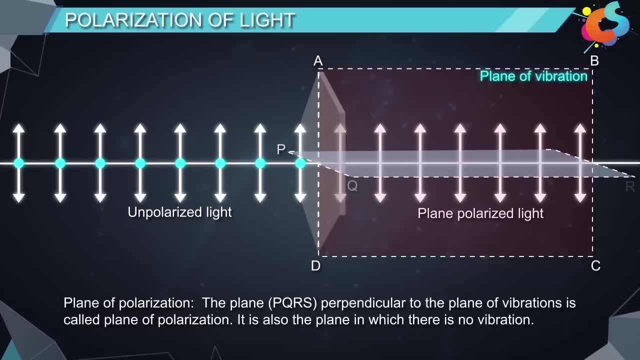 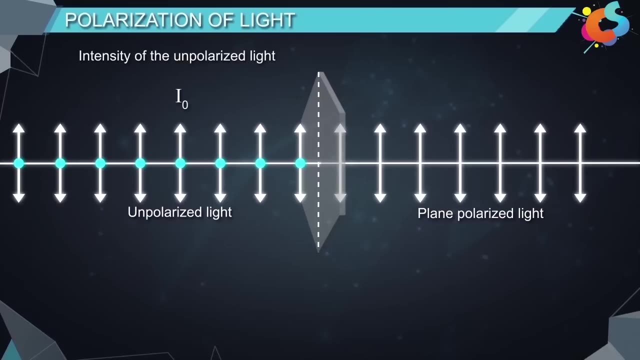 polarization. The plane PQRS, perpendicular to the plane of vibration, is called plane of polarization. It is also called plane of polarization. It is also the plane in which there is no vibration. If I0 is the intensity of the unpolarized light, then the intensity of the polarized light I coming out of the polaroid is given by: 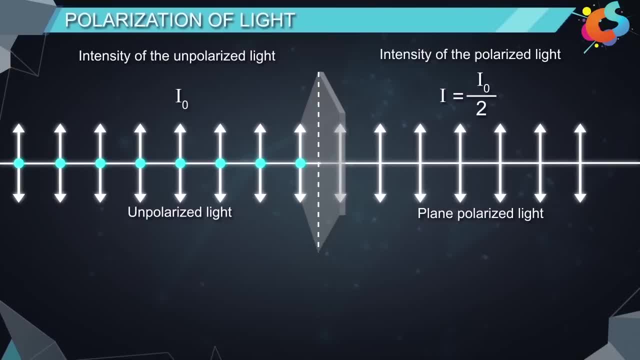 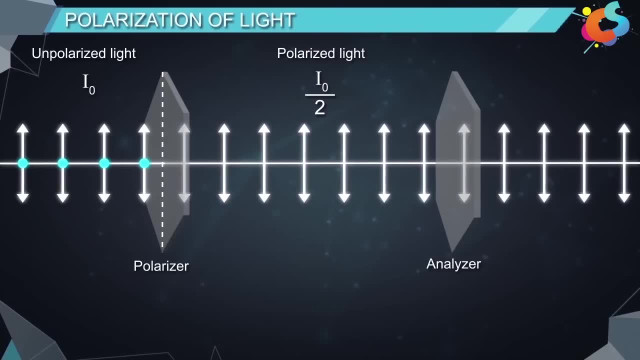 I is equal to I0 by 2.. Now if we pass this plane polarized light through another polaroid, we will call this as analyzer. If the pass axis of polarizer is parallel to the pass axis of analyzer, the emergent light will have no change in intensity. That is when theta is equal to 0. 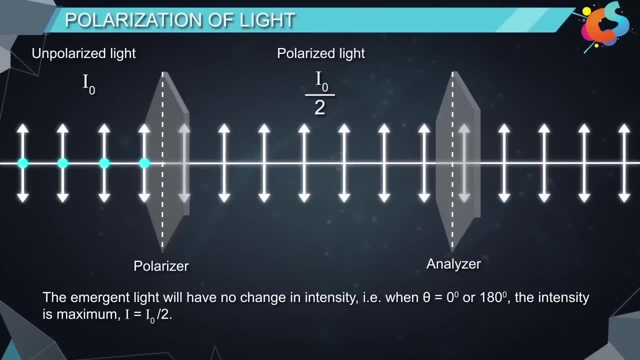 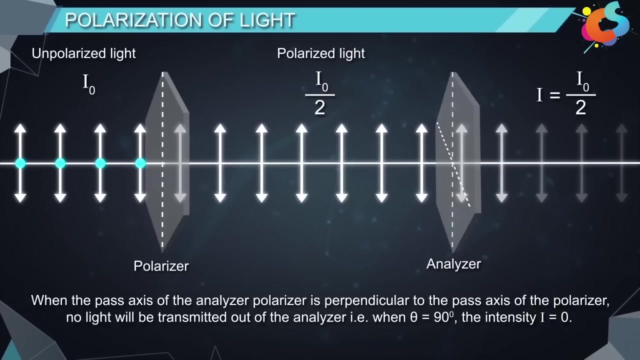 degree or 180 degree, the intensity is maximum, That is, I is equal to I0 by 2. I0 is the maximum intensity. If the analyzer is rotated by an angle, theta, then the intensity of the emergent light decreases. When the pass axis of the analyzer is perpendicular to the pass axis of the polarizer, 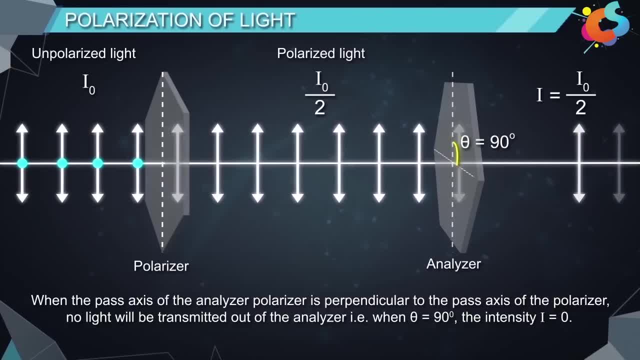 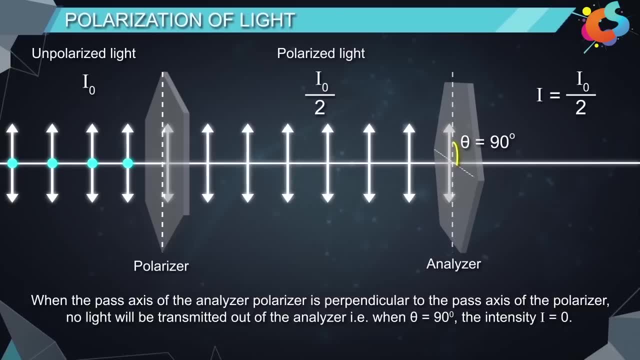 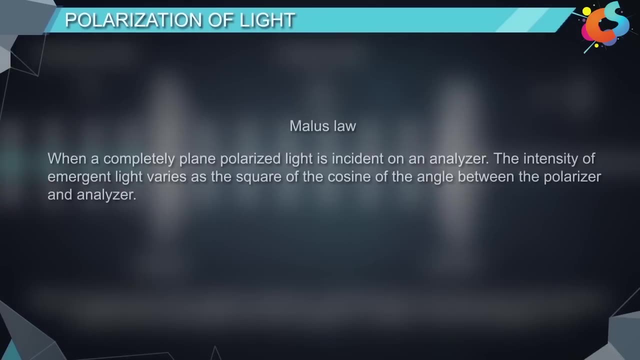 then no light will be transmitted out of the analyzer. That is, when theta is equal to 90 degree, then the emergent intensity I is equal to 0. Now Malus' law states that when a completely plane polarized light is incident on an analyzer, 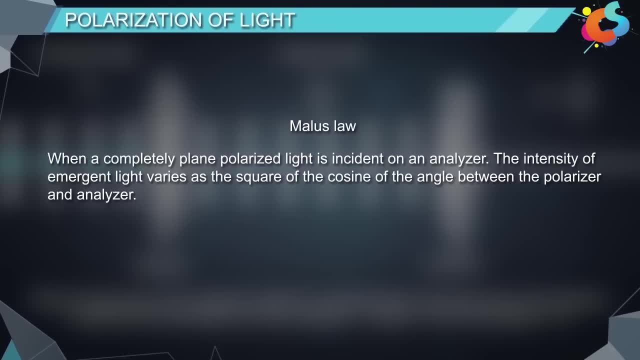 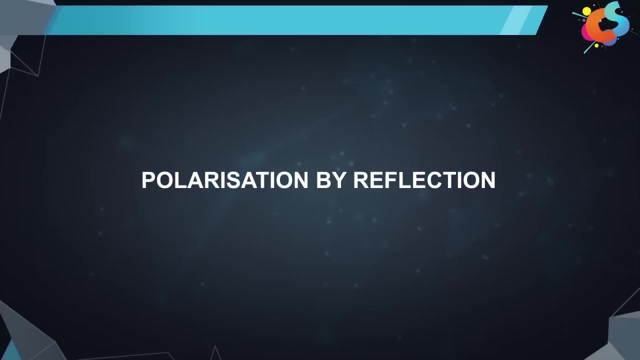 the intensity of emergent light varies as the square of the cosine of the angle between the polarizer and analyzer, That is, I, is equal to I0 cos square theta. Now I will explain the causes of unpolarized light: Polymerization by Reflection. 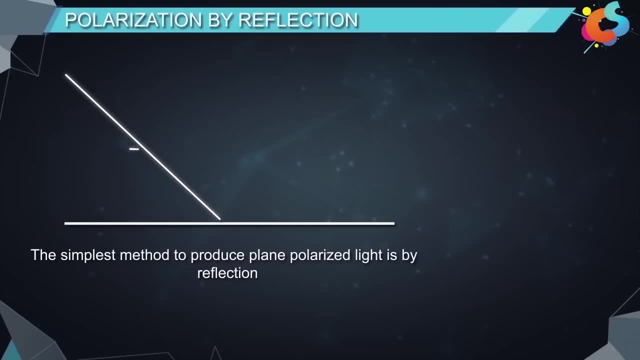 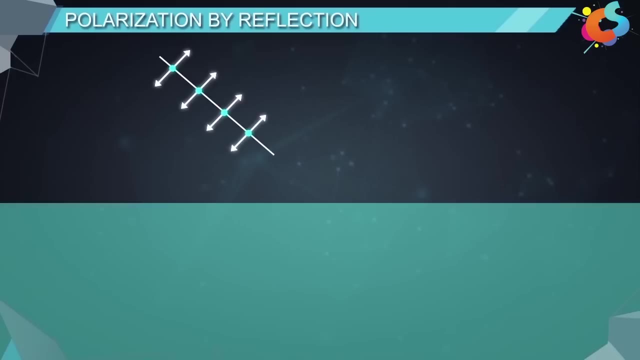 The simplest method to produce an unpolarized light is by reflection. This method was first discovered by Malus in the year 1808.. It was found that when an unpolarized light is incident on a surface of a transparent medium like water or glass, get Alsaci Some. 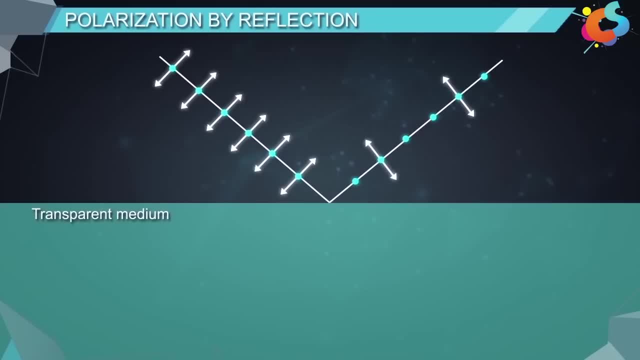 parts of the lens are in the tank, which then is fairly balanced and especially highly reflective. Some other parts are bedded, with only damages likeưỡbung and leadプولاريت. the light got reflected and the rest got refracted through the material. 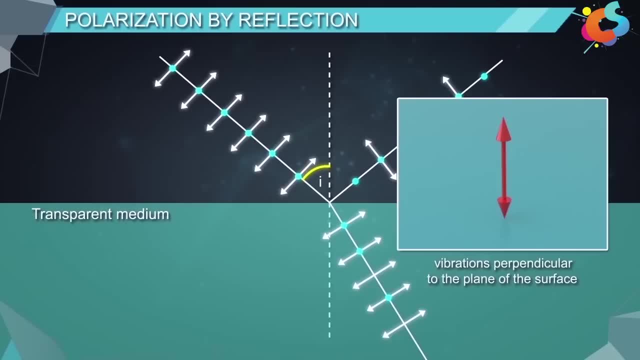 Here, the straight arrows represent vibrations perpendicular to the plane of the surface and the dots represent vibrations parallel to the surface. Now, if we observe the reflected light, we can see that it contains more number of dots than the arrows, which means that the reflected 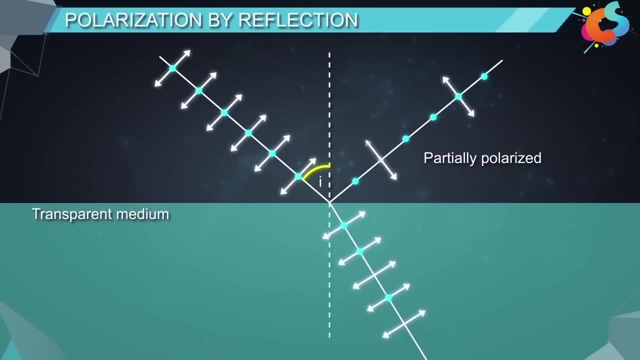 ray is partially polarized. Similarly, if we look at the refracted ray, we can see that it is almost unpolarized. It was found that as the angle of incidence changed, the degree of polarization of the reflected ray also changed Then at a particular angle. 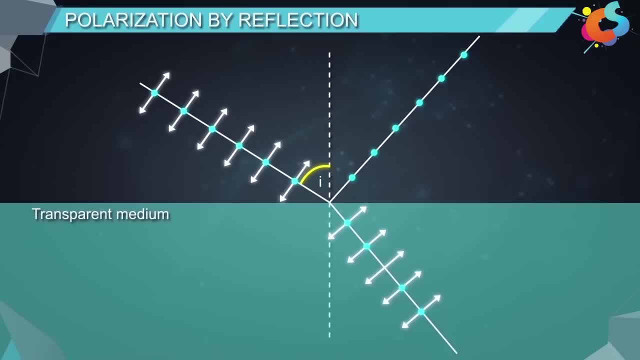 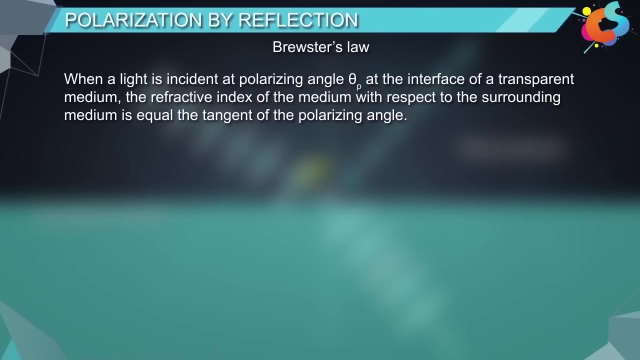 the reflected ray is completely plane, polarized, and the vibrations are parallel to the surface of water. This angle is called Brewster's angle or polarizing angle. Brewster's law states that when a light is incident at polarizing angle theta p, at the interface of a transparent medium. 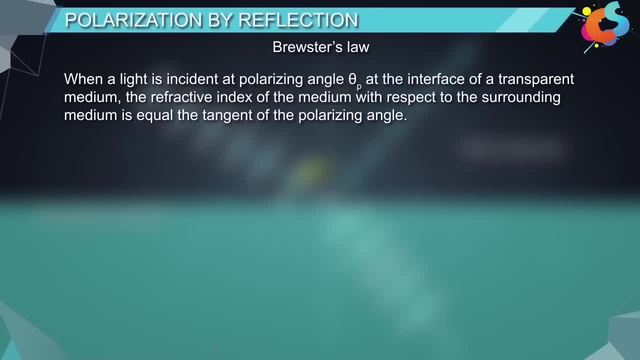 the reflected ray is completely unpolarized and the vibrations are parallel to the surface. refractive index of the medium with respect to the surrounding medium is equal to the tangent of polarizing angle, That is, n is equal to tan theta p, where n is the refractive index of the medium with respect to the surrounding medium.